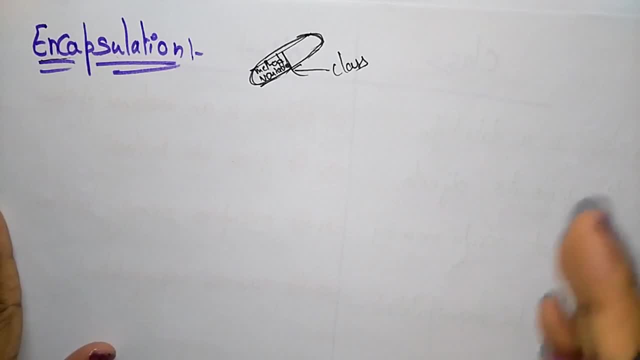 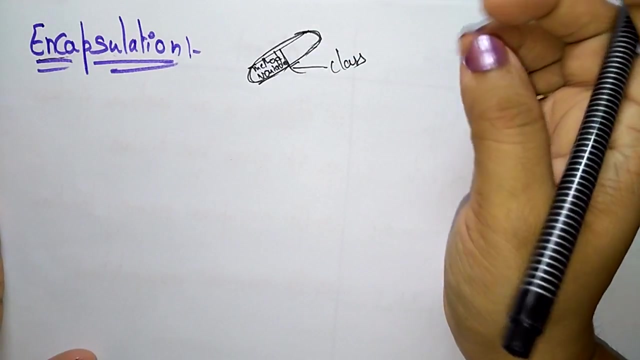 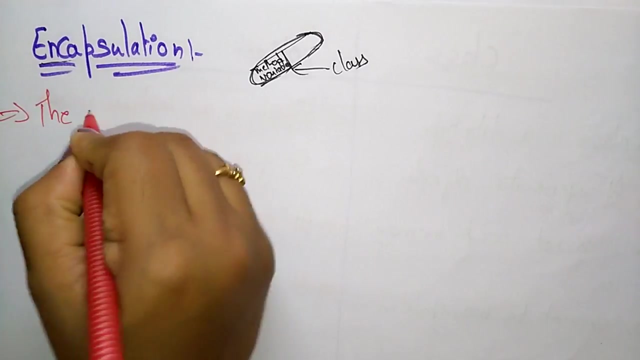 why we call it as encapsulation. So, if you want, if you are going to hide the data without showing to the means outside the glass, So it's just a wrapping of data. You call it as a encapsulation. So here the methods and variables of both are wrapped in a single unit that you call it as encapsulation. Let me write the definition for encapsulation. So this is one of the important topic. So while I'm explaining this encapsulation, please 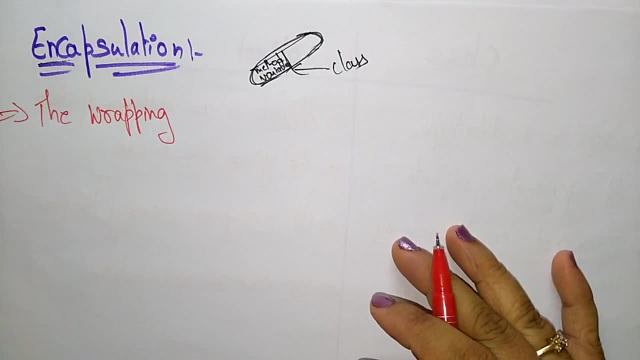 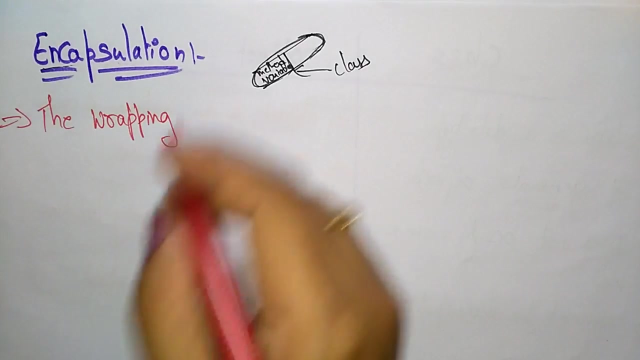 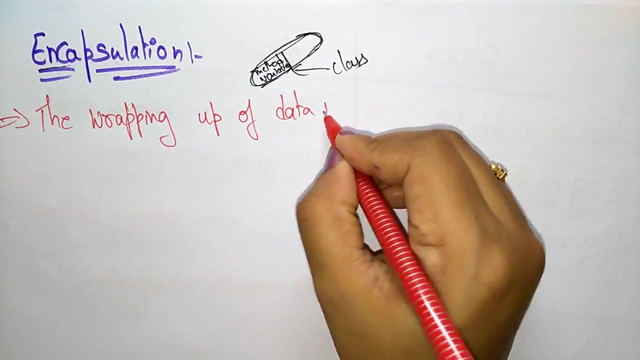 put concentration, because there is a small difference between encapsulation and abstraction, So don't be confused. What is an encapsulation, What is an abstraction? Afterwards I'll explain the difference between those two also, But try to understand what exactly the encapsulation was: The wrapping up of data. So here I'm. wrapping up of a data is nothing but the variables, The data and functions. that is a methods. 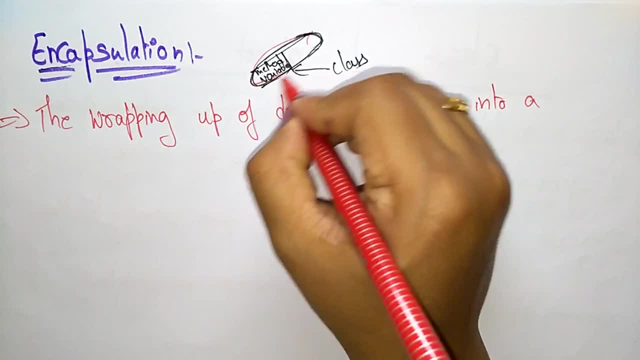 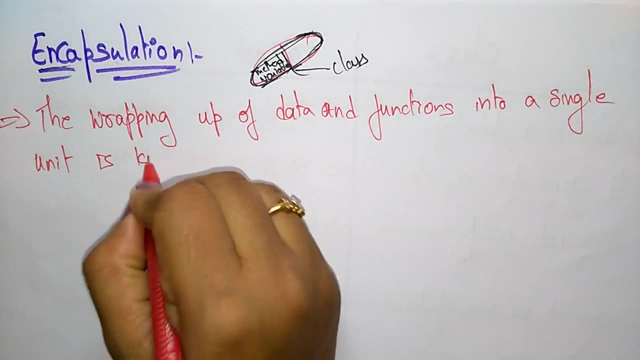 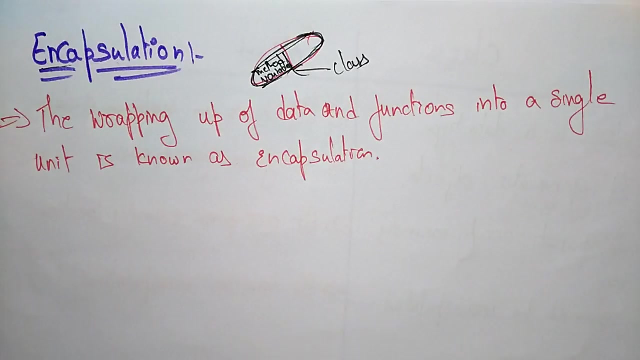 If you write elements into a single unit, So here it is wrapped in a single unit. So it is a rhetorical. that we're wrapping up data and functions into a single unit is known as encapsulation. So here it is saying that we are just wrapping the data and functions into a single unit is known as encapsulation, Even the classes also. wrapping the data into a single unit means a class is consist of data and the functions in the objects. You must be consistent in data and functions. So what happens then in a single unit? 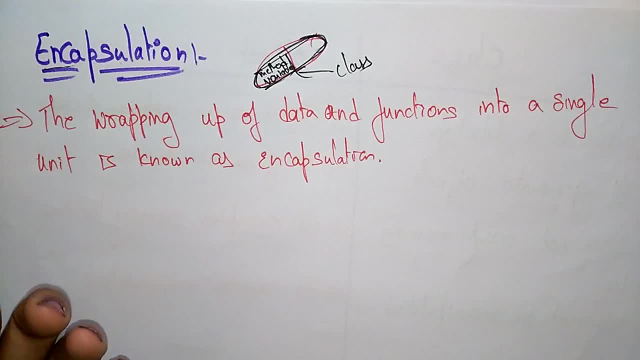 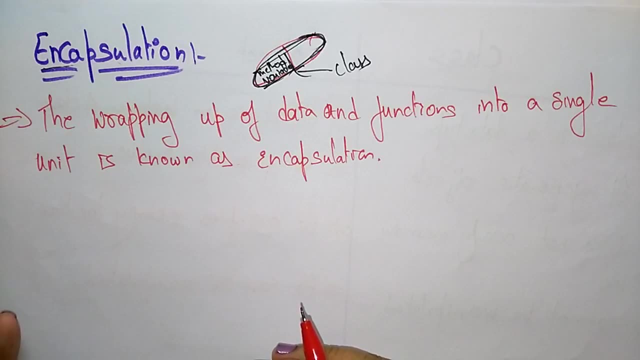 It says that in a single unit there are objects such that they cannot be wrapped into a single unit functions. so whatever the method you are taking, you are having means, the class you are taking there, the data and method will be there. then what is the difference between that class and 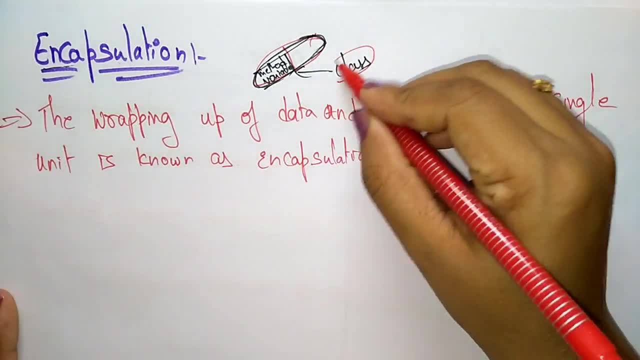 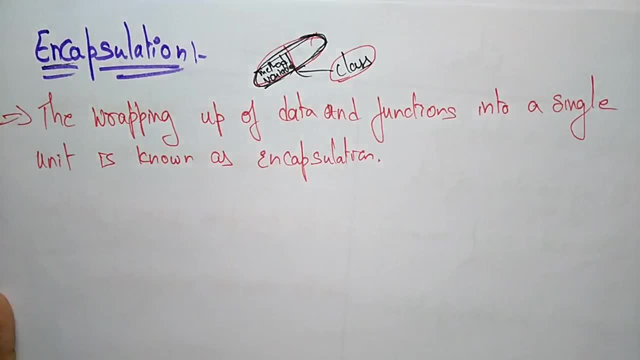 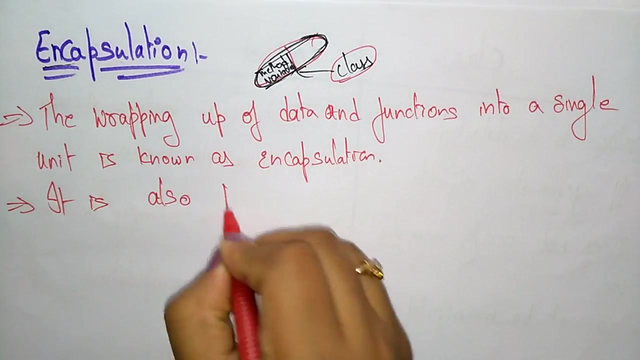 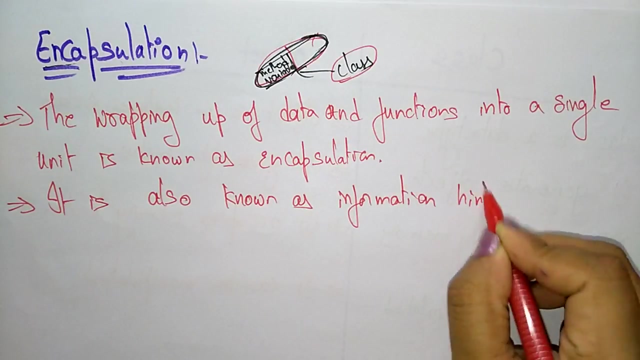 this encapsulation here. so here i am saying that the class is going to be encapsulated. how it is going to be encapsulated is wrapping up of data and functions into a single unit is called encapsulation, so it is also known as it is also known as information hiding concept. so here i added one more point, that is: 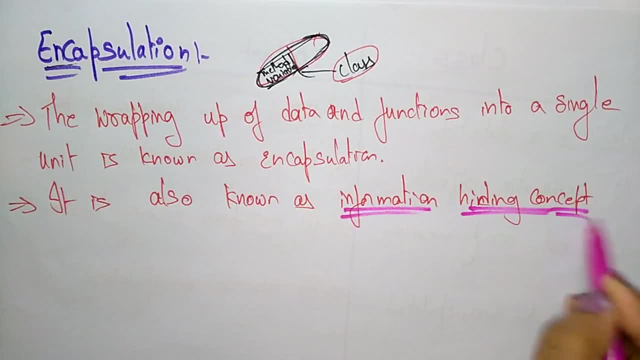 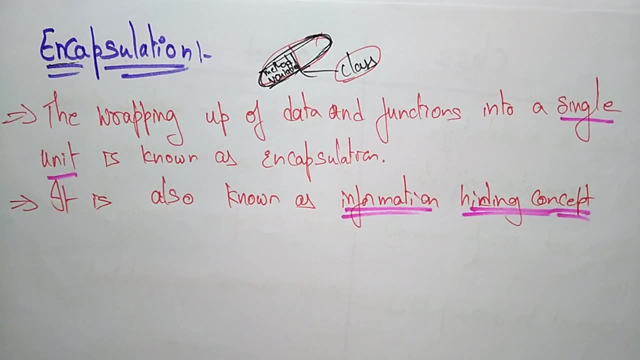 it is also known as information hiding concept. first i said it is a wrapping up of data and functions into a single unit. so after that i am saying that it is also known as information hiding concept. whenever i wrapped the data into a single unit, i said it is also known as. 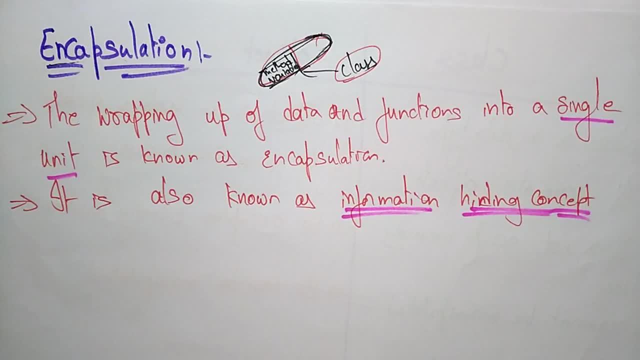 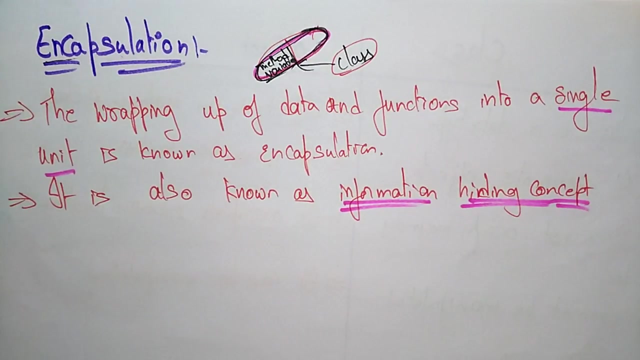 a single unit so that that data and functions are closed now just like a capsule, so in the capsule the data and functions are in a wrapped position, means in a closed. so that is why we call it as a information hiding concept. the encapsulation is a information hiding. 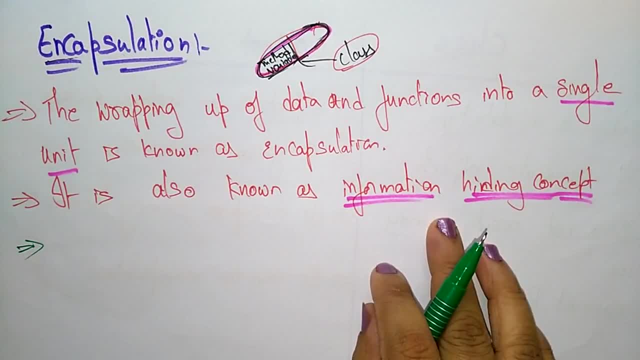 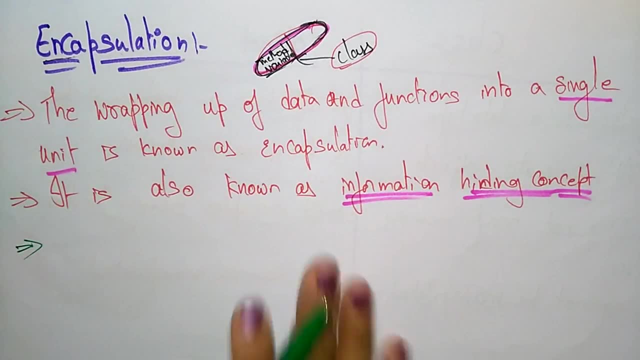 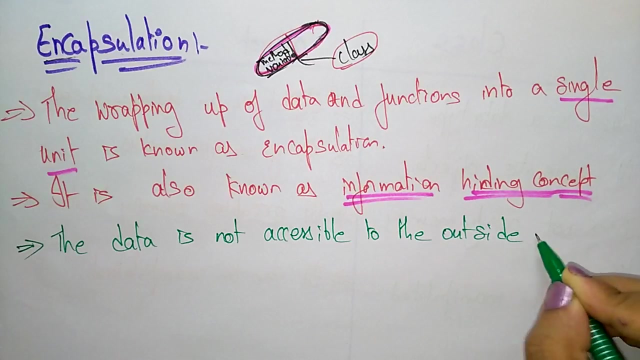 concept. so why it is information, why we say that it is an information hiding concept? because the data is not accessible, accessible, accessible to the outside world. let me write the point: because the data is not accessible to the outside world, because we are not able to see what is there in the 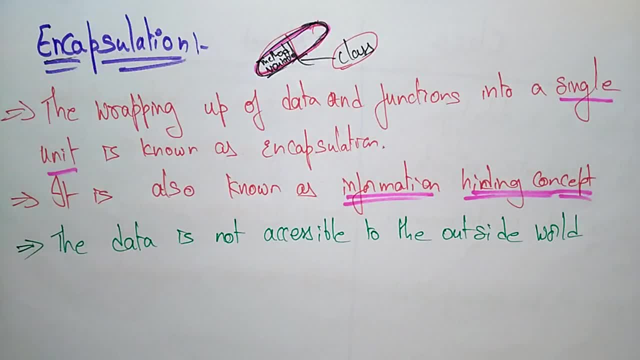 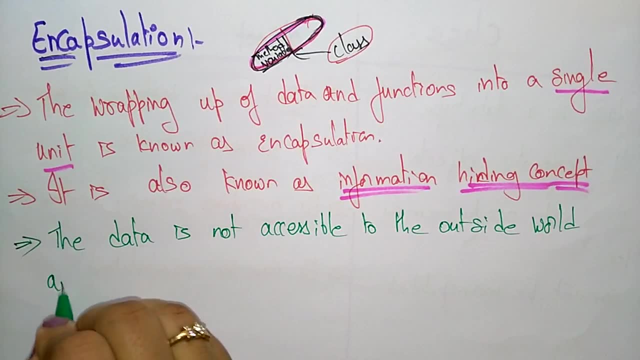 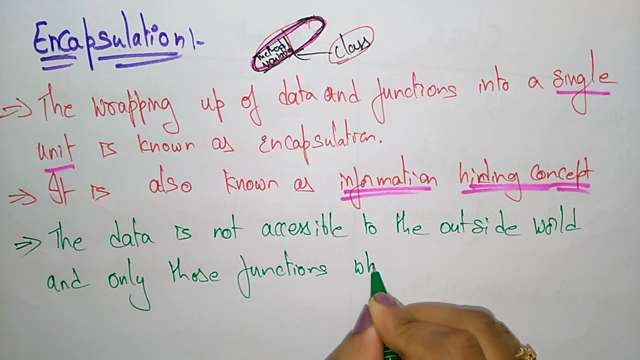 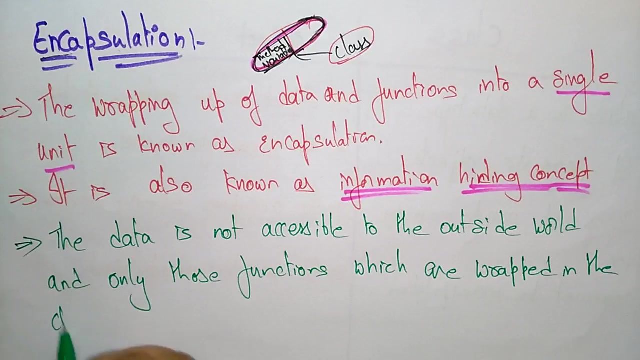 capsule. okay, in the capsule we know that some methods and variables are there, but we don't know what exactly it is present. so the data is not accessible to the outside world and only and only those functions which are rapid in the class can access it in the class can access it. so the outside world is not supposed to. 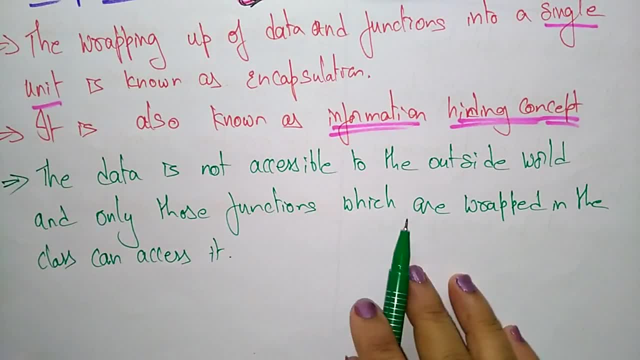 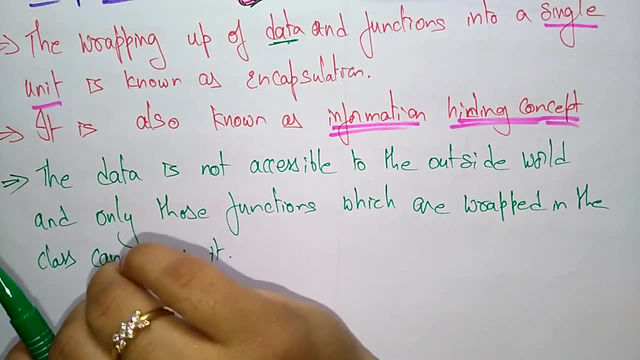 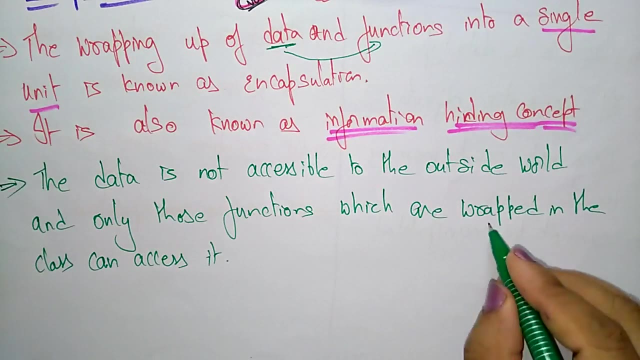 access the data and functions which is present in the class. so only those functions which are wrapped in the class can access. it means, whatever the data that is present in the club class, that data can access only those functions, okay, which are wrapped in the class. okay, so let 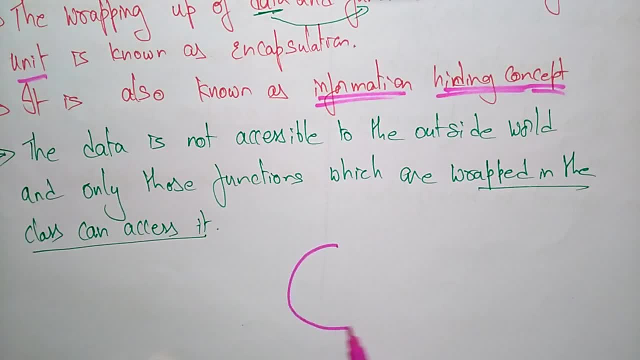 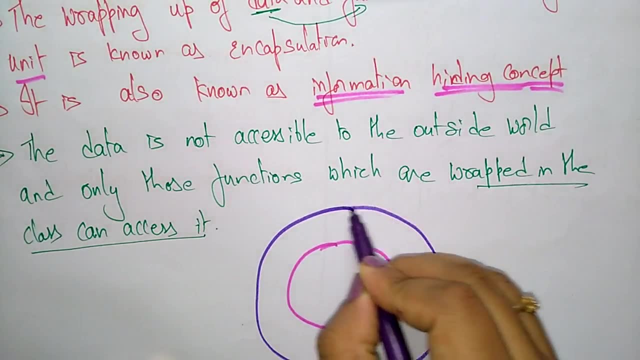 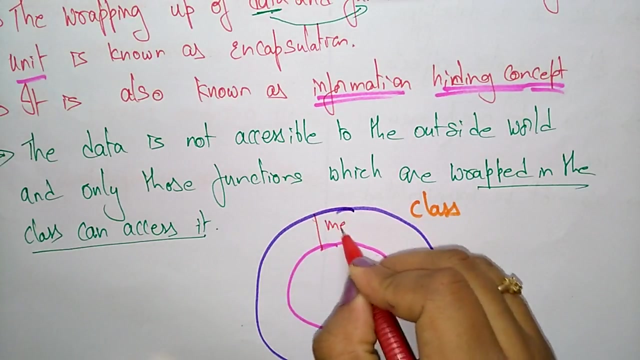 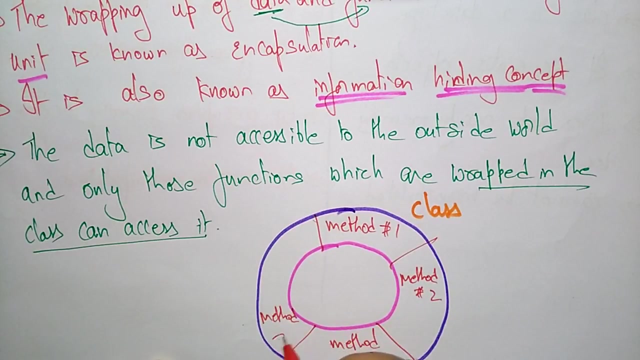 me explain with an example. so let us take: this is a data here, okay, and here the methods are there. this is a method, so this is completely. you call it as a class. a class is wrapped with methods. method one: let us take one. method two: so many methods are there. method three, method four and